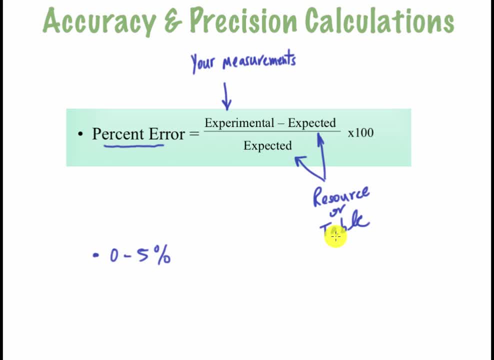 have to look it up in your book or somewhere else. It's going to come from a table or some sort of resource. okay, that is the expected quantity that you have in here. so experimental subtracting: uh, you know the expected. now one thing about percent error, because they're doing subtraction here, some people 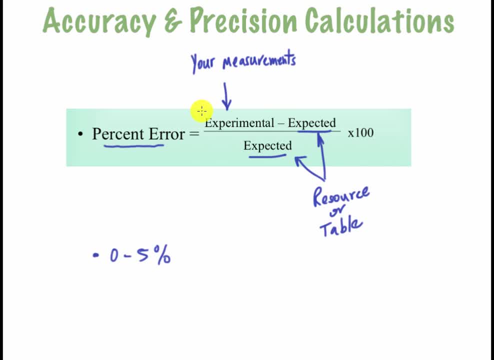 will do is some scientists, some chemistry teachers will put an absolute value in here. okay, it's fine, i get what they're doing, they don't. we don't want the negative, but i personally don't like that. i like the negative. so your percent error can be positive or it can be negative. the reason i like: 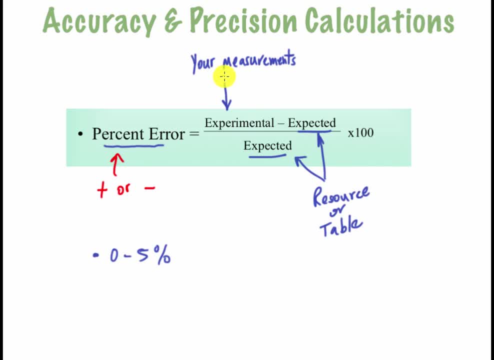 that is because if it's positive, then i know that my experimental measurement- my measurement- was bigger than what's expected. if it were negative, then i would know that my measurement were less than the expected. so this is really valuable information that it can tell you about what you need to do when you go back and look at it. all right, so let's take a look at an example. 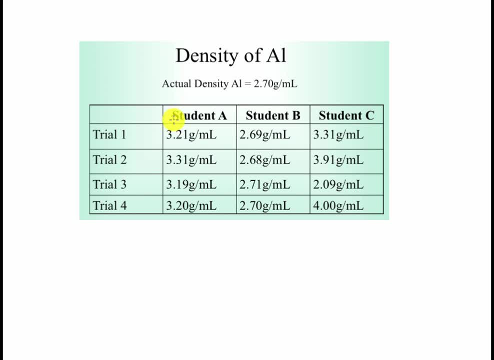 some example data. that is all right. so let's say we have a student here that's doing an experiment and they are trying to calculate the density of aluminum. okay, now here's the actual density. so this would be the expected amounts. that's what we would expect it to be and to be. 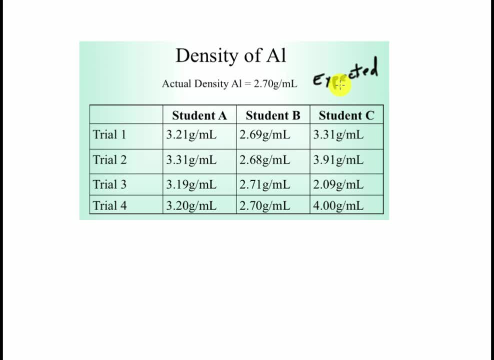 honest: in your labs you're not really doing experiments. you guys are doing labs, you're not. experiments will be unknown. what we're doing is we're just practicing skills and comparing it to the known things that scientists have already figured out. you're not going to discover new things in here. 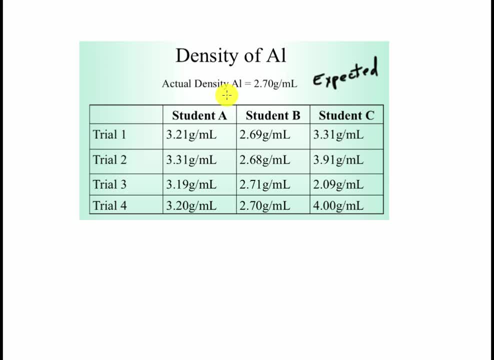 unfortunately. if you do, let me know, because you can make some money on that. but for now, we're doing is really looking at comparing our data, our calculations, our measurements to actual accepted things. so you're going to see a lot of this expected stuff. all right, so this is what it should be. we take a look. 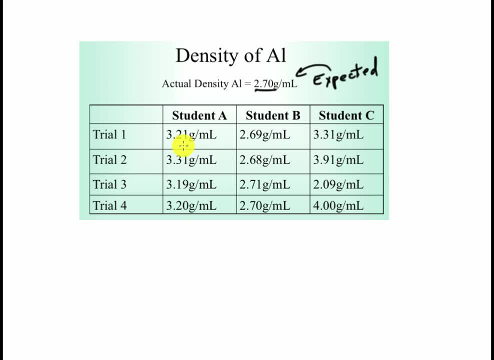 at student a student a's data for four trials- 3.21, 3.31, so on. very precise. that data all looks very similar. right, they're all pretty close to each other, but the level of accuracy is not quite there and we can do and to figure this. 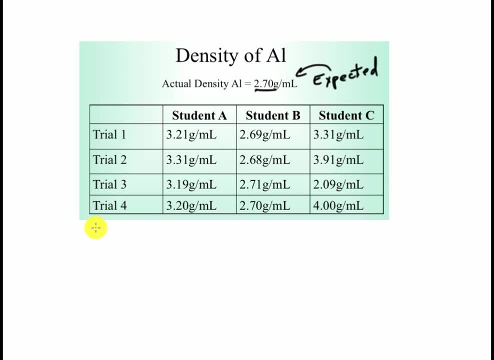 out we want to look at is the average. so we can do is we can say: student a's average data, right? so this is what you're going to do when you guys are doing a lab and you have a student a's data and you have a student a's data and you have a student. 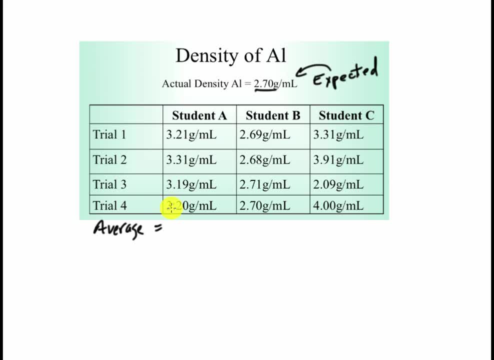 a's data and you have four or five trials, we're not going to look at each one individually. what we do is we average all of those trials. so we're going to do is: because each trial was exactly the same, you didn't do anything different for trial one than you did for trial four. we're going to add them up. 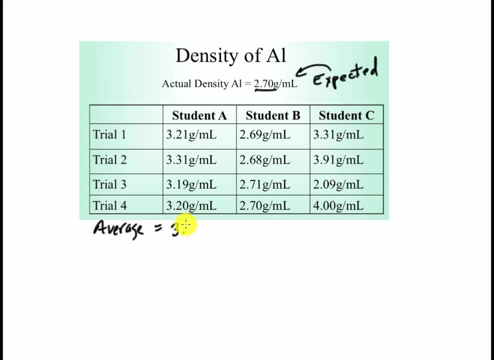 and divide by four. when you do that, you get three point two, two, seven, five grams per milliliter. okay, so that would be the average value for student a's work. now again, don't forget about significant figures. you're gonna have to round this to the correct number of significant. 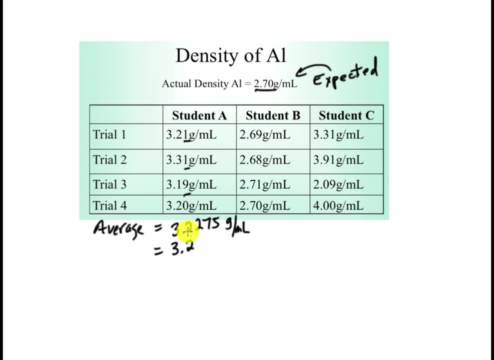 figures and, based on the fact that we're at least this decimal point here, we're gonna go ahead and divide that out by with three significant figures. my final answer. so I should end up with three point two: three grams per milliliter. if you're still having questions on that, please ask a. 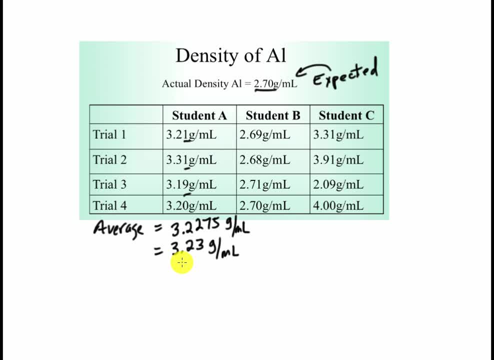 significant figures can be a little crazy in the beginning, so please make sure you get some help in that. on that in class, alright, so that's my average value. obviously it's not not close to the two point one. I guess it's close. it's it's closer than four, so it's doing a little better here. by the way, take a. 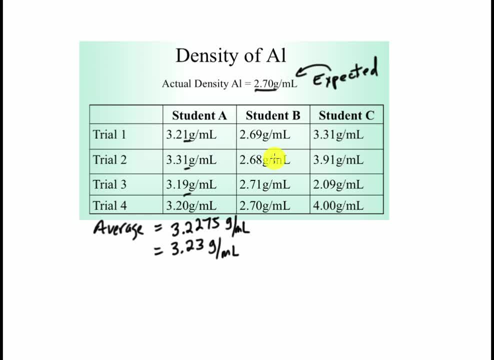 look at student C's work: very, very sloppy. this is the kind of thing I'm looking for. student a: good, okay, I'll accept that. student B: awesome, very, very good, you're right on track. student C: what's going on here? I mean, this is just sloppy. you should not be getting this. you know your measurements. that are all. 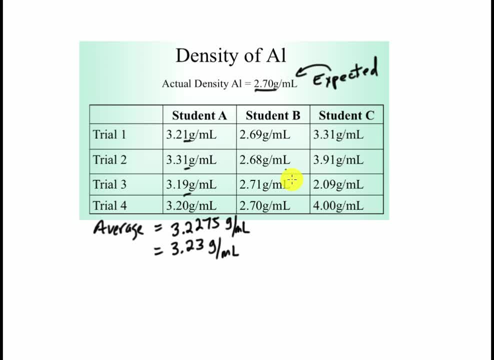 over the place. you know there's no precision, there's no accuracy here. student B: precise and accurate. student a looks very precise but not quite accurate. so let's figure out how far off the mark that's going to be for student a student is, and that's where we do our percent error. okay, so we'll do our. 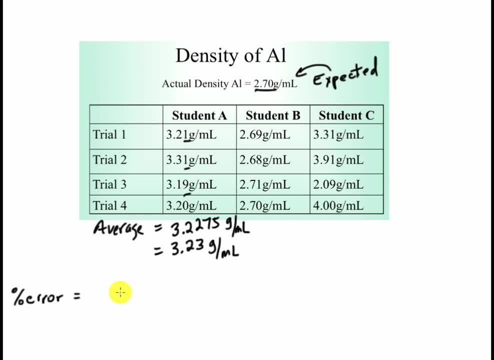 percent error calculation here, which would be the experimental, which is what we hear, with the student measured. so this is from the experiment, from what they determined. so three point two, three grams per milliliter minus the expected. okay, so we expected that to be two point seven, zero grams per milliliter. you. 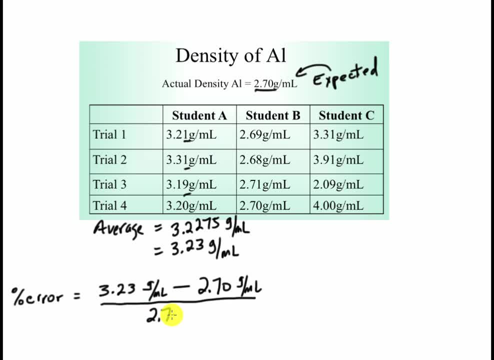 divide that all out by two point seven zero grams per milliliter. when we do this, we do the subtraction, what you're gonna end up with is a value of point five, three grams per milliliter. okay, over two point seven zero grams per milliliter. so I 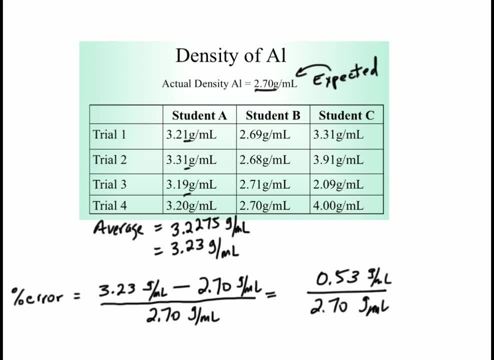 haven't done the math, I'm just doing it step by step here. the reason I'm doing this? just to show you some more with the significant figure. so I'm significant to the second decimal place. to the second decimal place. since I'm subtracting, I have to round this to the second decimal place, which is what it happens to do. 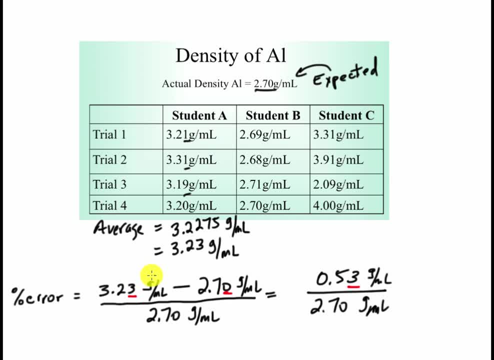 when I do the subtraction. so three significant figures, three significant figures. I now have two significant figures in this number, okay, so by doing this subtraction I've actually lost some significant figures here. I still have three significant figures in the bottom number. okay, so I'm using my rules. 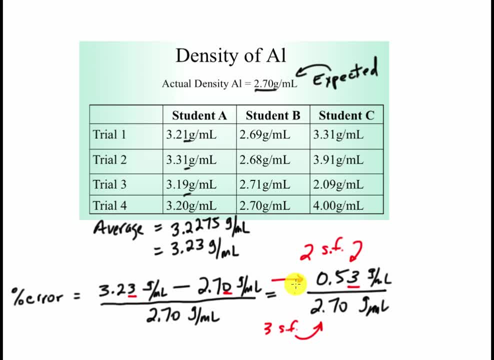 applying the rules for subtraction here to get that number here. now I'm gonna follow my rules for multiplying and dividing. when I divide, I have to count the number of significant figures. since I have two significant figures here, I have to put two in my final answer. so when I do the 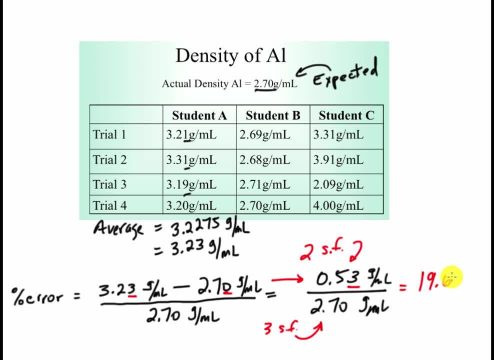 calculation, I get nineteen, point six, two, nine. well, I can't round there because I have to do three significant figures and three significant figures ends on one, two, three on the six. okay, so from it. oh, I'm sorry, not three significant figures, I need two, so we actually have to round it at the nine. okay, so two significant. 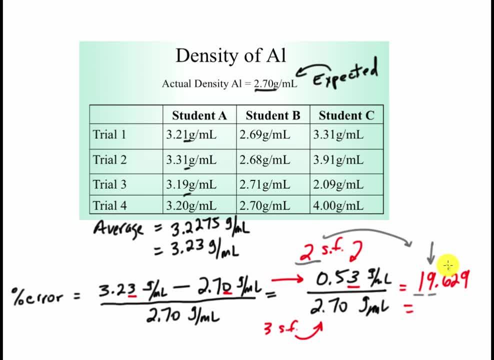 figures here at the last number, and then the last number is the decimal, and the decimal and the decimal here is a C, so I have to round this up to a twenty and I have to put a decimal here because I want to show that this is a significant 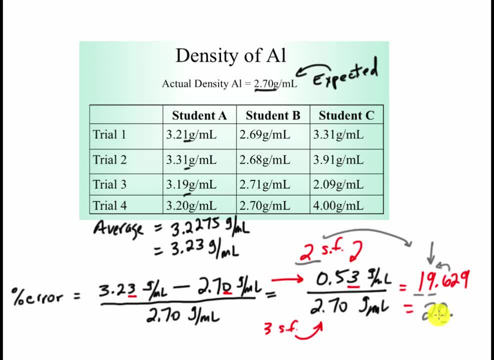 this is the hardest one, guys. I know that these are confusing. are those trailing zeros? why I chose this? to kind of make it look, give you an example of this. alright, so, because the answer is 20, if I don't put the decimal here, then it's.